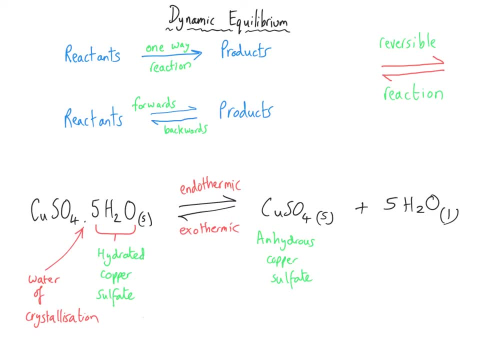 that when you add water to the anhydrous copper sulphate, the temperature is going to go up, And that is a characteristic of any reverse reaction. So what is anhydrous copper sulphate? Anhydrous copper sulphate is an anhydrous copper sulphate. 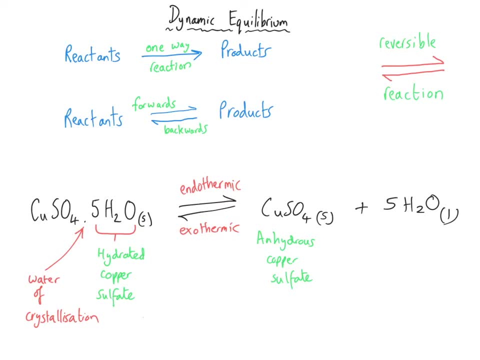 It's a reversible reaction. One of the directions will be exothermic and the other will be endothermic, by the exact same amount. it's just one of them. the energy will go up, one of them. the energy will go down. It doesn't have to be backwards is one and forwards is the other. 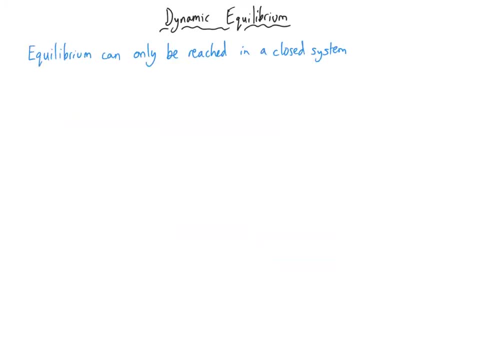 it can totally vary. Now, equilibrium can only be reached in what is known as a closed system And if you remember from the energetics video, we discussed that that is where anhydrous copper sulphate can be reached. And if you remember from the energetics video, we discussed that. that is where anhydrous copper sulphate can be reached, And we need to design a neue situation that results inذا steps. we need to transform subtraction into a resultant- resultant. So if we were going to back this equation up and try to get this equation- till its real position back seríaeking a lemon key. it brings exactly the same assumption that something is possible in x, y, k. aliment Bidersermej тому elıs bag is equal to same as vu segu ATy in seus terrenos finali. emssi en sus heros. 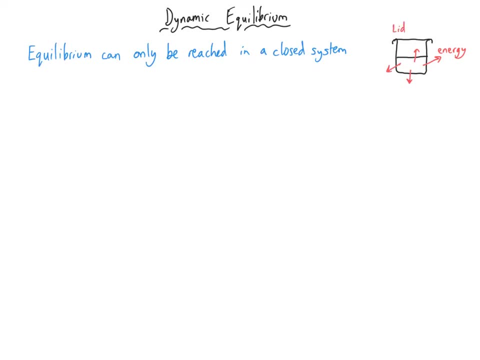 That can be as simple as having a lid on a beaker so no gasses can go in or out, And conversable reactions are usually referred to as existing in a state of dynamic equilibrium, And in fact that could be a two mark question where you're asked to define what a dynamic. 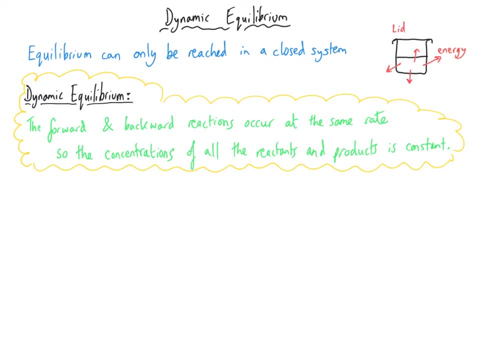 equilibrium is. So there's obviously two parts to the answer. So the first part is that the forward and the backward reactions are both occurring at the same rate, And that's the origin of the dynamic part of the definition, that the forwards reaction is happening and the backwards reaction is happening. 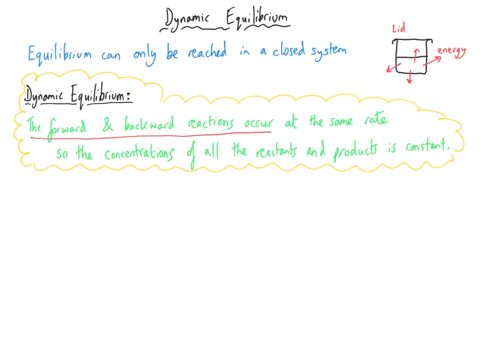 Now the equilibrium part is really sort of like a twofold part to it, The fact that it's at the same rate. that's one aspect of the word equilibrium. And then the other aspect of the word equilibrium is that the concentrations of all the reactants and products is constant. 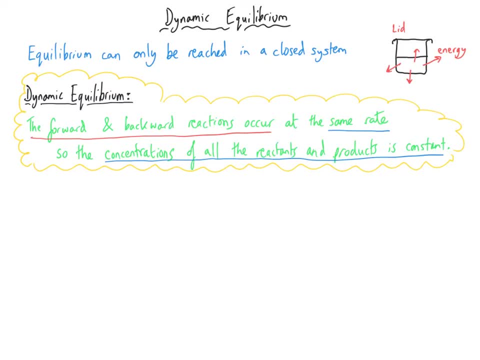 And so you might not have the same amount of both, but the amounts that you have of reactants and products is unchanged. Now, the best way of visualising this is actually to look at a graph. If we look at a typical graph of a one direction reaction, where reactants turn into products only, 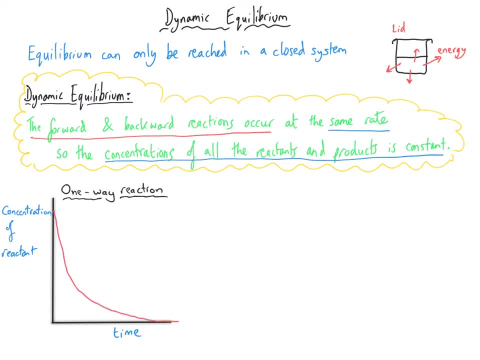 over time the concentration of reactants will obviously decrease as the reaction goes on. It decreases really quickly at first, then begins to slow down, and then it stops when one of the reactants or both of the reactants or all of the reactants have been used up. 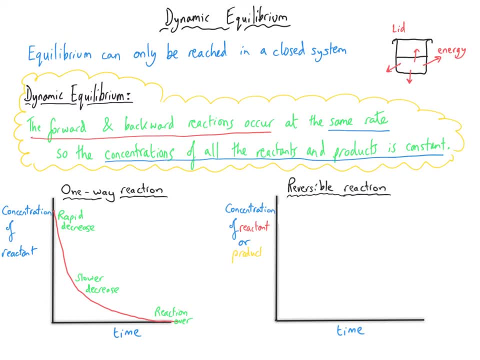 However, in a reversible reaction, that is different. If we look at the concentration of the reactants, that follows the same sort of path of decrease, but over time it decreases more slowly until the point where it levels out, and it doesn't level out at zero. 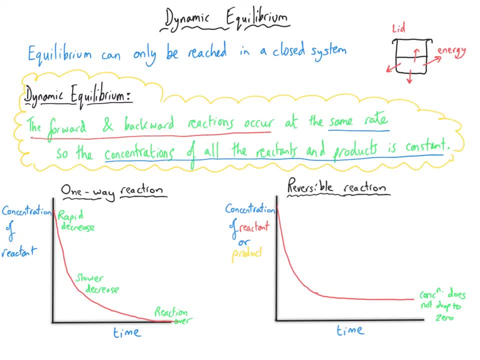 Who knows exactly where it levels out, but it's definitely not zero. There is definitely some reactants left over. If we were to map the concentration of products in the same sort of way, then obviously at the beginning of the reaction we have zero concentration of products. 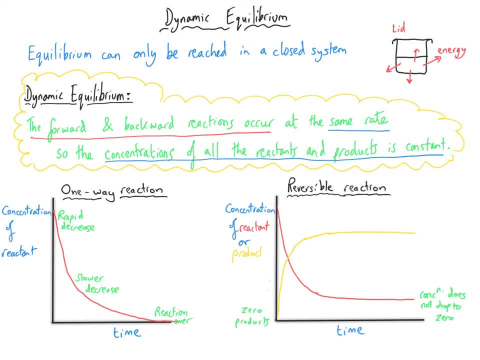 Quite quickly. we make some products and then the rate of making of products decreases because the amount of reactant that we've got left over has decreased. So the rate of the forward reaction is going to slow down. So we're going to make less product and then, after a time, 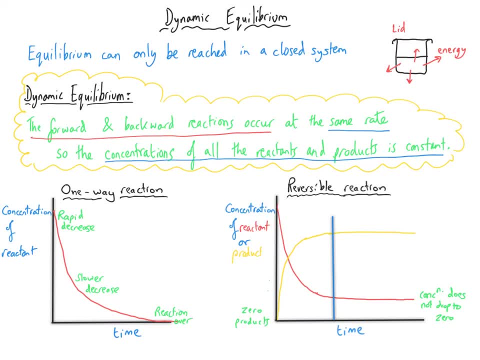 the concentration of products will level out and not change any more, And that coincides with the same place where the reactants doesn't change any more. And this is the point that equilibrium has been reached. Now, to repeat, it's a dynamic equilibrium because the forwards and the backwards reactions are both happening. 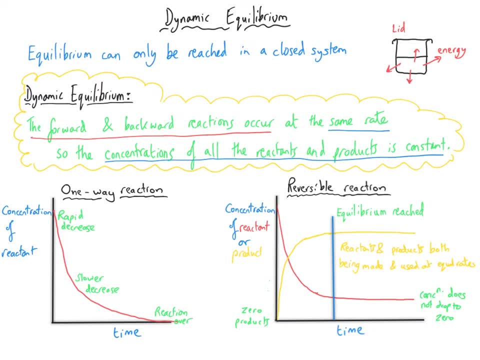 but the concentrations of the reactants and products. they have no overall change because the product is being made at the same rate that the reactant is being used And because the reaction is reversible, that product is being used up at the same rate that it is made as well. 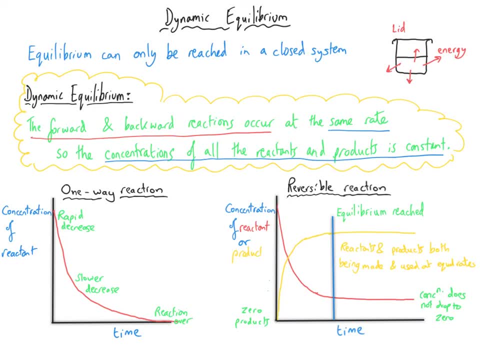 and reactants are forming again. So overall, the reactants and products, whilst they're both being made and used, there is no overall change. Now the position of the equilibrium is very rarely 50-50.. There's no easy way of looking at an equation and working out what the position of equilibrium is. 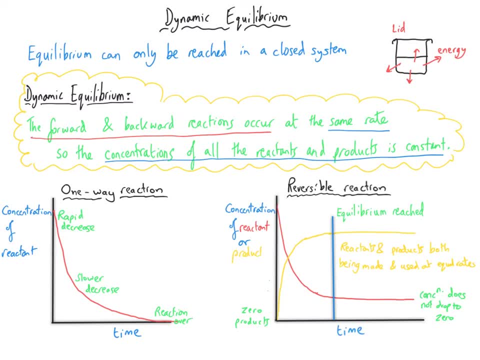 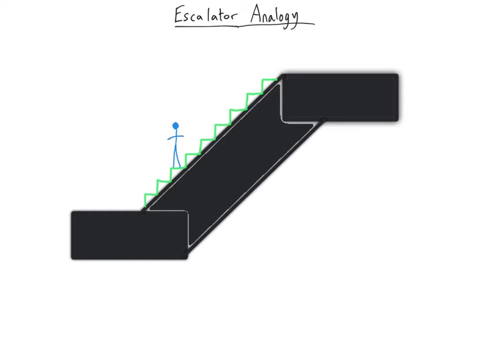 You can actually only tell whether there are more products than reactants by doing an experiment to find out how much of one of the reactants or products you've actually got. More on that later Now. a really good analogy for a reversible reaction in dynamic equilibrium is an escalator. 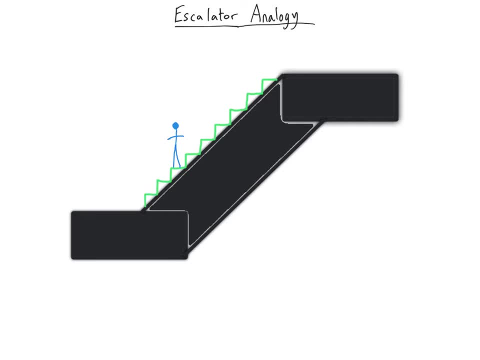 Now escalators, the moving stairs that you don't have to walk. whilst they are taking you in one direction, they will move and you will move with them, And so this is moving downwards. Now, obviously, you shouldn't, probably for health and safety reasons. 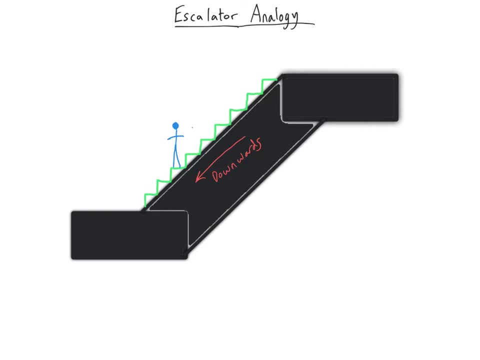 but probably everybody does. you can go against the escalator, So you can go upwards on a downwards escalator And if you run fast enough you will get to the top and even though the escalator was trying to take you downwards, 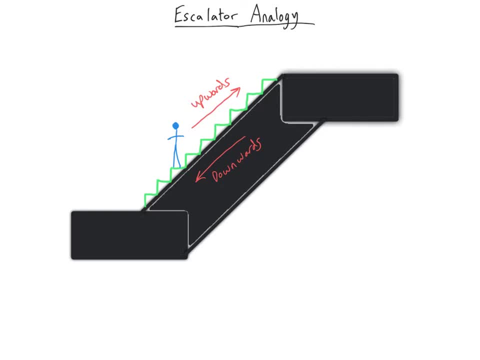 the upwards won because the upwards was at a faster rate. However, you will, if you're clever, be able to match your upwards walking to the downwards movement of the escalator, And here you have reached equilibrium, You've reached balance. 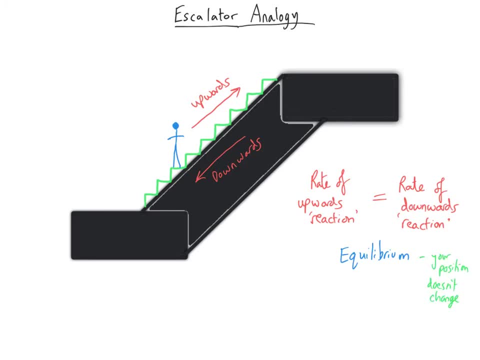 because your position, up or down, won't be changing. You will be effectively still, whilst also moving, And that's why it's called a dynamic equilibrium: because you are moving, your legs, your muscles, your muscles are working and the escalator is working. 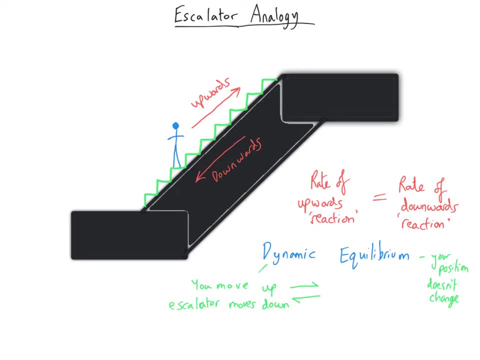 so the upwards and the downwards are both happening, but your height is not changing because you have reached equilibrium And you could do that at the bottom where we've got here. so three steps up, or you could do this three steps down. 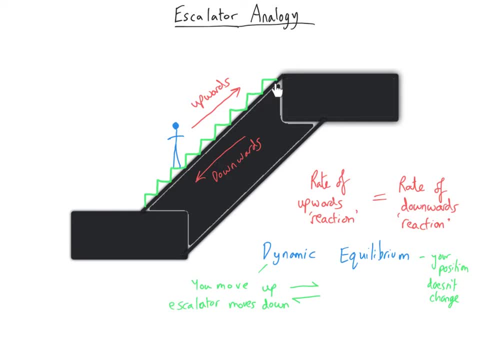 You could do this in any position up or down on the escalator Equilibrium, that position of not actually moving your overall height, your height not changing. you could do this three steps along the escalator, Just like a dynamic equilibrium might be 90% product and 10% reactant. 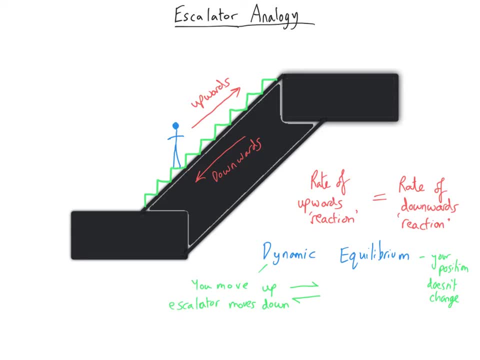 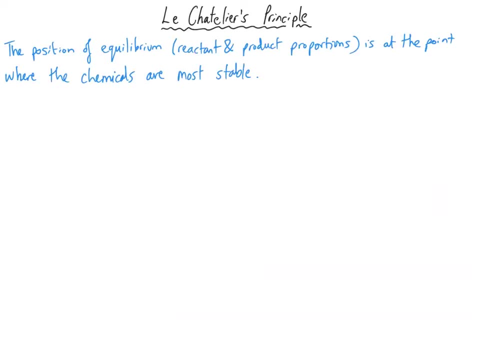 or any other combination. So that's a really good analogy. You can reach equilibrium whilst walking up a down escalator. I just mentioned that the position of equilibrium could be 40-60, could be any proportions at all- And so I wanted to begin. 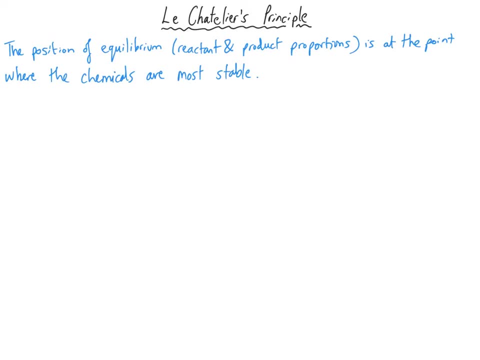 this section by looking at what it is that affects that proportion. And so the position of equilibrium- and that means the proportions or the ratios of reactant to product- is at the point where the chemicals are most stable, And the fact that they're the most stable at this point, 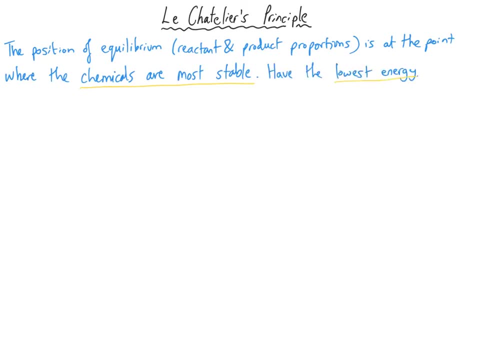 means that they have the lowest energy, And at that equilibrium, there will be a certain set of conditions, and these conditions will be to do with an optimum temperature, pressure and any other factors that might happen to be affecting the chemical reaction. Those conditions are such that they: 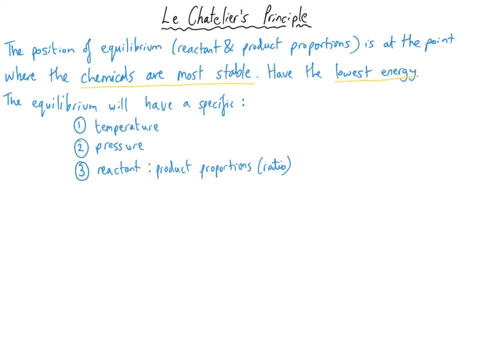 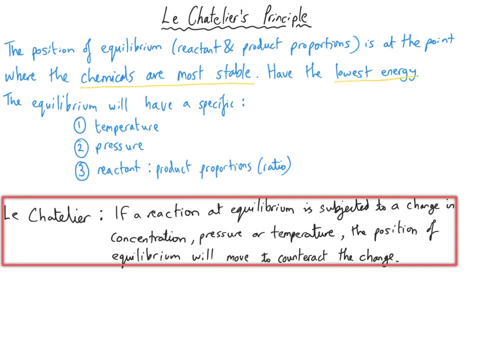 are in the most stable temperature, for instance, as well, And so Le Chatelier's principle states that if a reaction at equilibrium is subjected to a change in concentration, pressure or temperature, the position of the equilibrium will move to counteract the change. 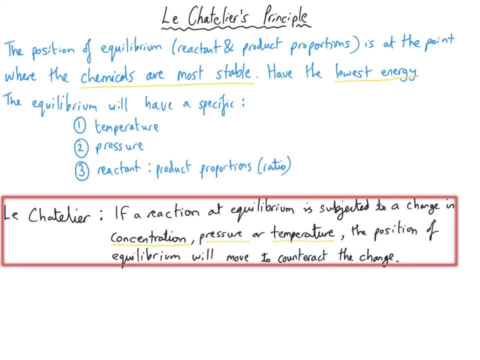 Which is really fancy sounding, but you know he was a professional scientist and he wanted to sound clever. However, we can reduce that definition down to something that's more usable, which is that equilibria shift to oppose change And those few. 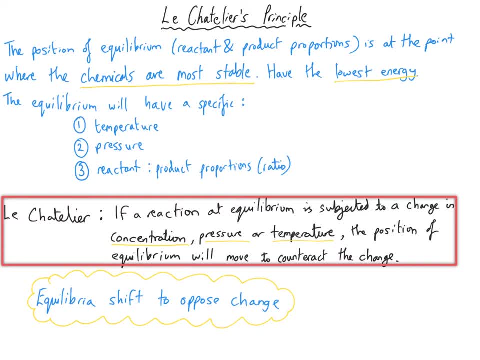 words are really powerful, particularly for your understanding of Le Chatelier's principle, And even in exam situations. it can help your approach to any number of types of questions about equilibria, And we should be absolutely clear here the reason that the equilibrium 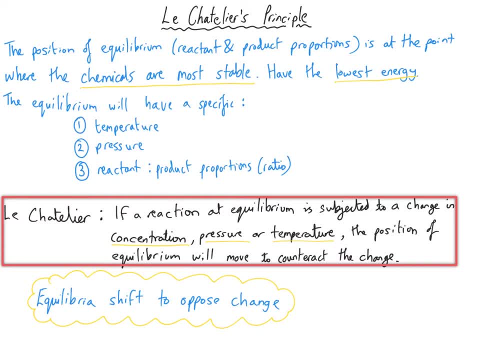 is shifting to oppose the change is not through any conscious thought. The equilibrium is not something that we can personify. It is doing it to maintain stability. So if we impose a change upon it, that makes it less stable than before And the equilibrium 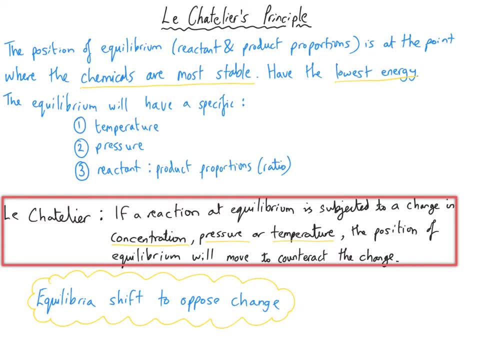 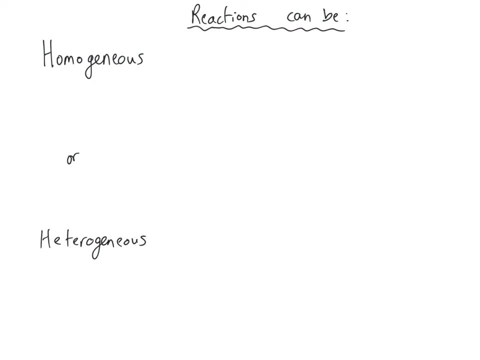 shifts spontaneously to become as stable as possible. Before we explore Le Chatelier a little bit more deeply, I just want to clarify two terms about chemical reactions. Now, chemical reactions can be described as homogeneous or heterogeneous. Now, actually heterogeneous are a little. 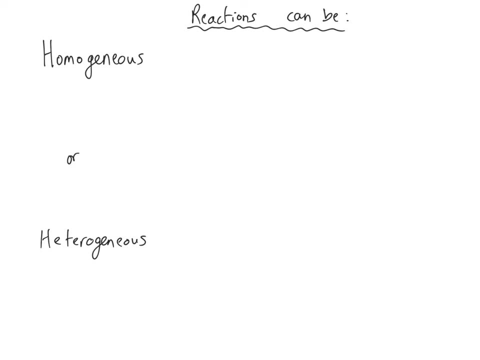 bit more common than homogeneous. but in terms of equilibria, you're only concerned with homogeneous equilibria situations. Now, a homogeneous situation is when all the reactants and products are in the same state And normally they're all going. 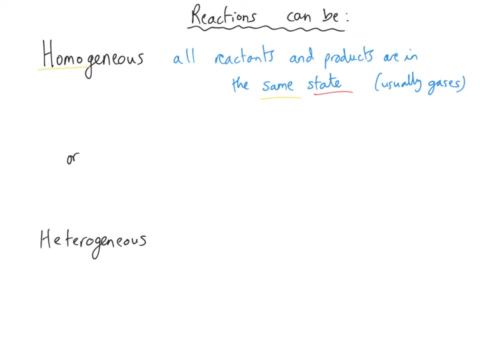 to be gases, And so that's derived from homo, meaning the same, and genius is what links it to state, And it would follow that heterogeneous meaning hetero being different and genius still being state. so all the reactants and products. 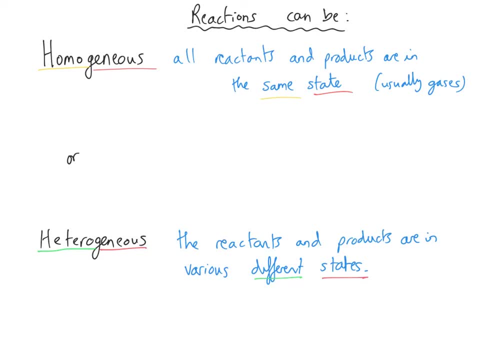 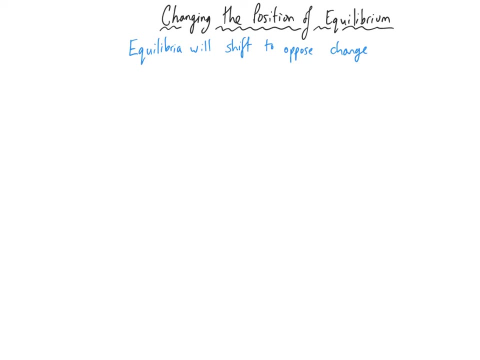 could be in a variety of different states, so they aren't all in the same state. So Le Chatelier tells us that anything that we do to an equilibrium will be opposed by the equilibrium itself shifting, And so what that means is, if we increase the temperature, 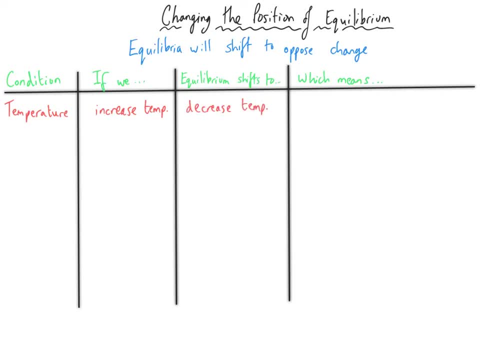 equilibrium will shift in the direction that lowers the temperature, And that is the endothermic reaction. If we decrease the temperature, equilibrium will shift to oppose that, to raise the temperature up again, And that will be the exothermic reaction From the point of view of pressure. 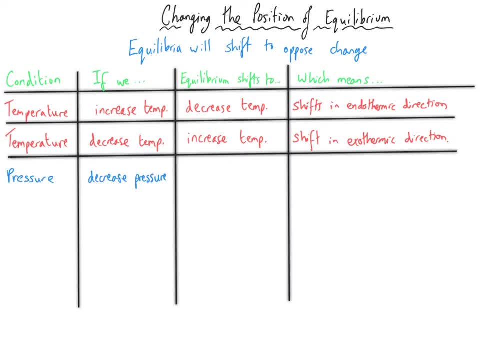 if we decrease the pressure, equilibrium will shift to raise the pressure back up again, And the higher pressure is the side of the reaction that has got the greatest number of molecules of gas. And if we raise the pressure, equilibrium will shift to lower the pressure back down again, And that will 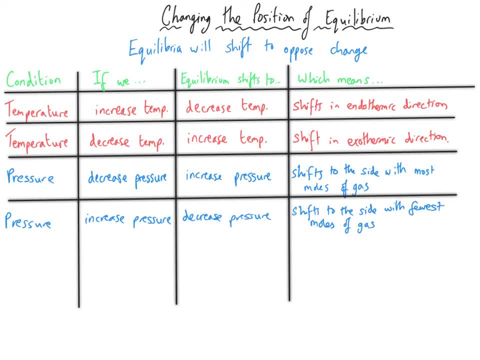 mean that the reaction will shift in the direction where there are fewer molecules of gas. And finally, if we increase the concentration of a particular chemical in the equilibrium, the equilibrium will shift in the other direction to decrease the concentration of that reactant or product. 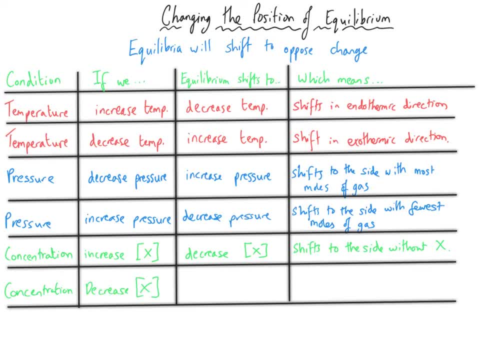 And it follows that the exact same thing is true if you were to decrease the concentration of a particular chemical, the equilibrium would shift to increase its concentration, to make more of it, and that means it would shift to the side that has got that particular chemical. thereby 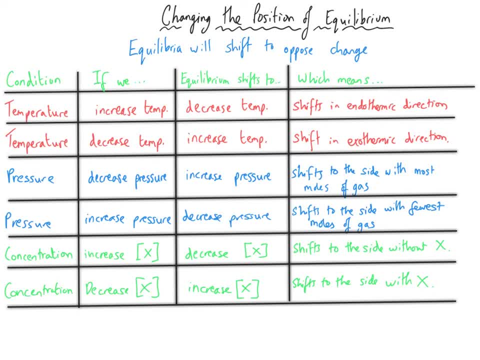 making more of it to restore that most stable of conditions, which is what all of these shifts are to do. Now is probably a good time to point out that the square brackets around a particular formula, such as square brackets around x, means concentration of chemical x And that 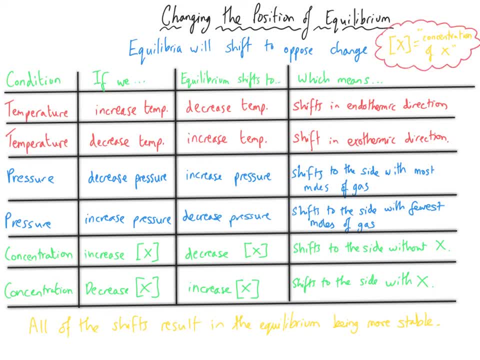 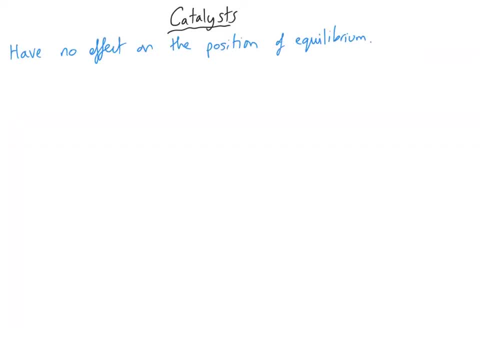 is just a shorthand notation for that, which definitely makes things a bit faster and is totally fine to do in an exam situation. Now, I haven't mentioned catalysts until this point, and the reason that catalysts are less significant is that they have 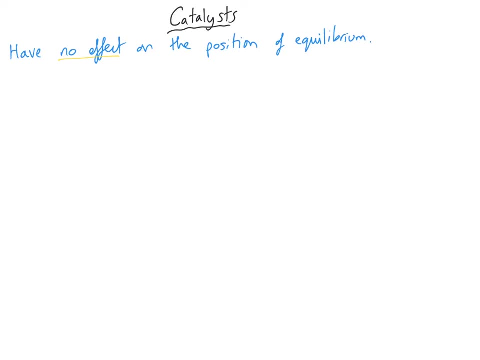 no effect on the position of equilibrium. The reason that this is true is obvious if you consider a reaction profile. So if we have a look at an exothermic reaction profile in the forwards direction, you can see why this reaction maybe is reversible because the 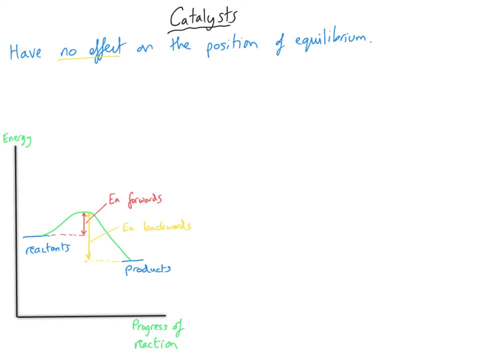 energy barrier. the activation energy in both directions is not particularly big, which is what allows both the forwards and the backwards reactions to happen. However, what catalysts do is they lower the activation energy and if you consider the reaction profile, the activation 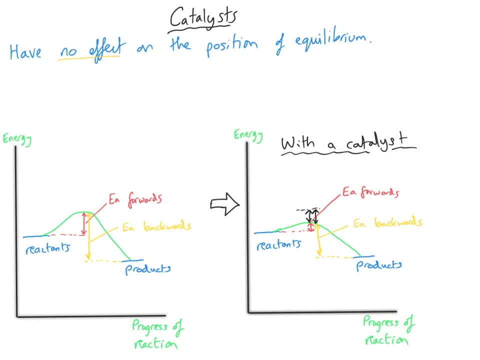 energy gets decreased by the same amount for both the forwards and the backwards reaction, because the hill just kind of gets lower, so to speak, And so the forwards reaction and the backwards reaction will be sped up by equal amounts, And so all that would happen 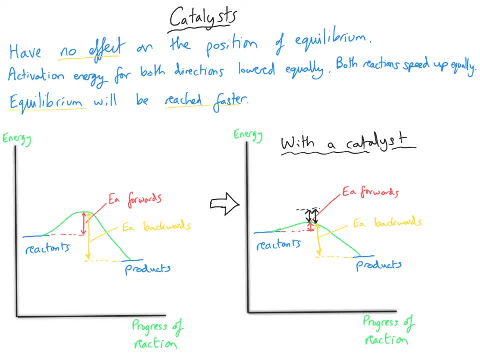 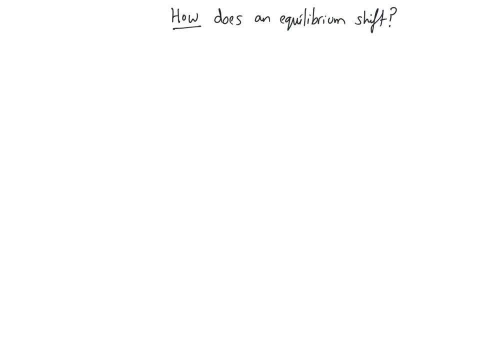 is, equilibrium would be reached faster. A question that you are probably asking is: how does an equilibrium actually shift? And the answer is that it shifts by speeding up in one direction. So if we consider first of all a system that is at equilibrium, the rate of the 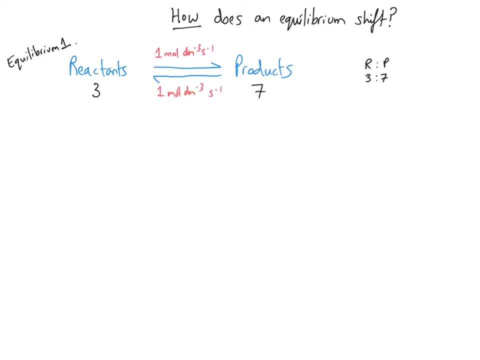 forward and backwards reactions are the same. Let's say that they are one mole per decimetre cubed per second. If an equilibrium shift happens, say in the forwards direction, so it shifts to the right hand side, then the forwards reaction will increase Maybe. 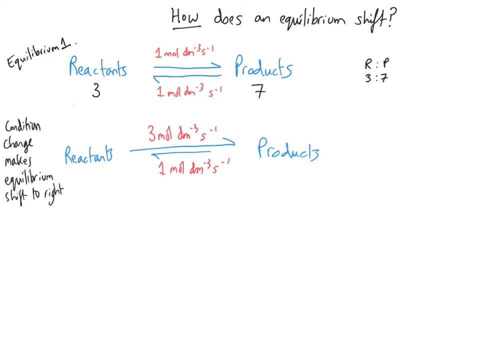 its rate of reaction will increase to three moles per decimetre cubed per second, And at that point of increase the forward reaction is faster than the backwards reaction. So that means that we're making more product than we have been making reactant. 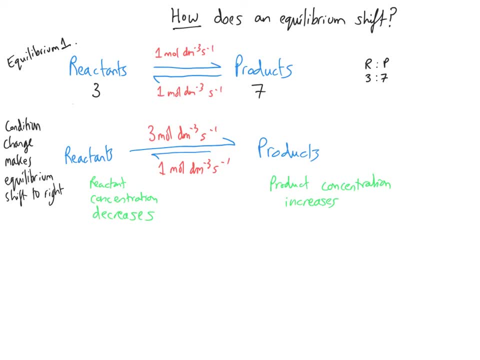 And so the position of equilibrium, which previously was three to seven in terms of the proportions of the reactants to the products, has now increased to two to eight, But because we've now got more product and we've got less reactant. 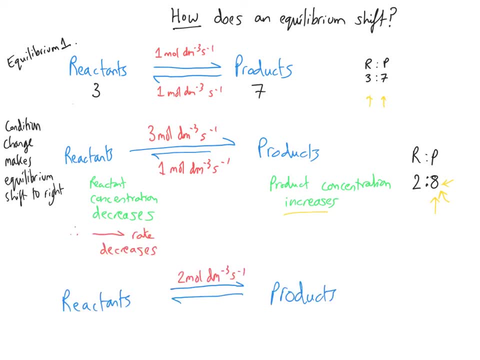 the rate of the forward reaction decreases down to, say, two moles per decimetre cubed per second, and the rate of the backwards reaction increases from one mole per decimetre cubed per second up to two moles per decimetre. 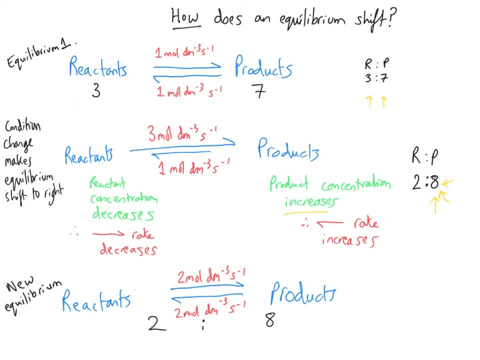 cubed per second. And so now we have a situation where the forwards and the backwards reactions are equal again, Different rate to before, but they're equal again. And so now, from this point onwards, the concentration of the reactants and products will. 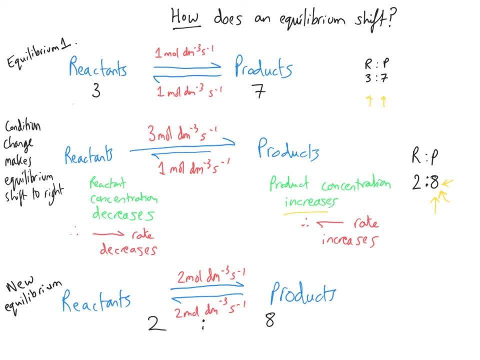 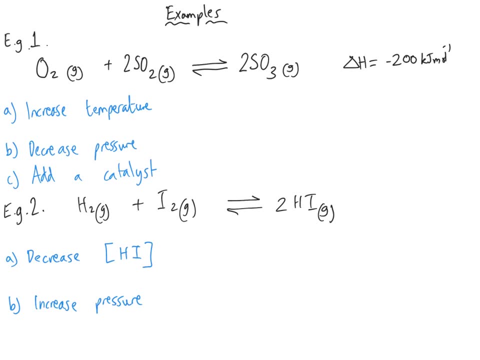 remain constant, Even though it is still dynamic. the reaction is still happening. Let's take a look at a couple of examples of equilibria and how they would be affected by the changes that we've outlined here. So in the first example we've got oxygen and 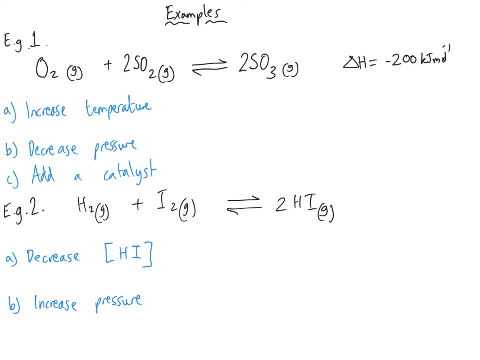 sulphur dioxide, producing sulphur trioxide, and the delta H is minus two hundred, which we need to take a moment to process as meaning it is exothermic, And that's really important. for this first question. If we increase the temperature, equilibrium shifts. 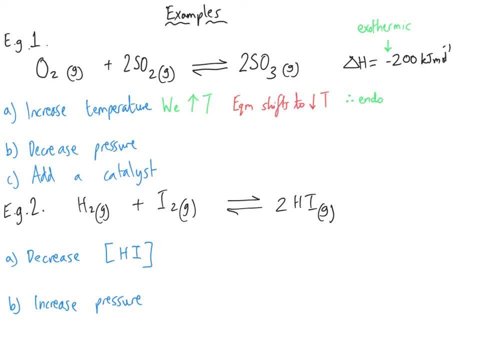 to decrease the temperature, which is in the endothermic direction, so to the left-hand side here. So equilibrium shifts to the left-hand side. For part B: if we decrease the pressure, equilibrium shifts to increase the pressure, and so it shifts. 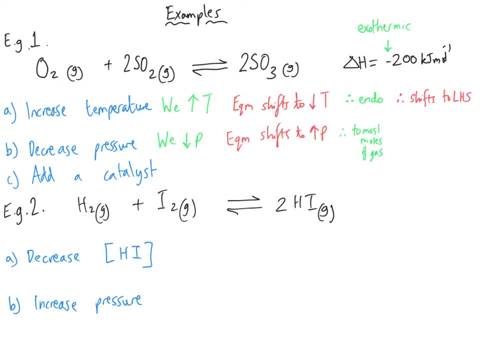 to the side with the greater number of molecules of gas, And there are three on the left-hand side and only two on the right-hand side, So the side on the left-hand side is the higher pressure side and so shifting to the left, which is what happens. 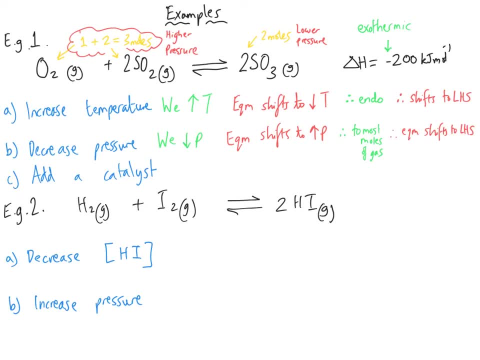 has the effect of increasing the pressure. And finally, adding a catalyst. well, that's a trick. Adding a catalyst has no effect on the position of equilibrium at all. Onto the second example. If we decrease the concentration of hydrogen iodide gas, 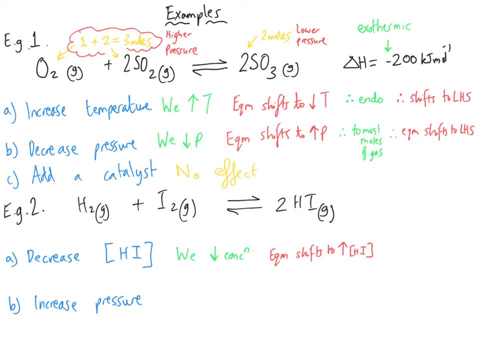 then the equilibrium will shift to replace it, to make more of that hydrogen iodide gas, to try and restore the balance of concentrations, to reactants, to products, And so that means it will shift to the right-hand side. And then the final example of increasing the pressure. 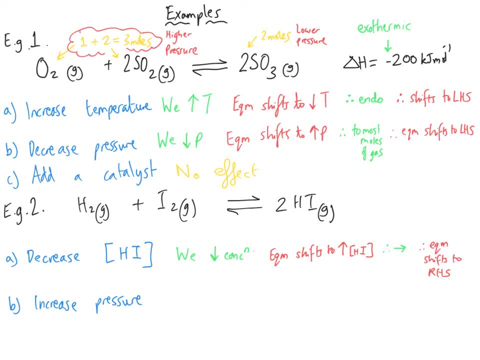 Well, equilibrium shifts, if it can to decrease the pressure. Now it can't actually do that here, because there are two molecules of gas on the left-hand side and two molecules of gas on the right-hand side, So the pressure of both sides. 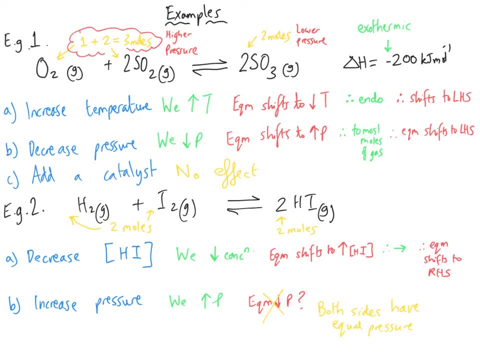 is equal, and so increasing the pressure or decreasing it, in fact, would have no effect on the position of equilibrium, although, it should be pointed out, it would affect the rate of reaction. We're going to finish this video off by looking at some industrial. 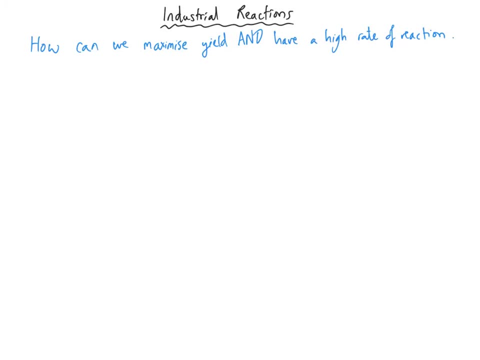 processes and looking at how we can maximise the yield of a particular target chemical whilst not really putting the rate of reaction under any negative impact. Unfortunately, this isn't always possible and it's really important that you can appreciate that sometimes we have to have a compromise. 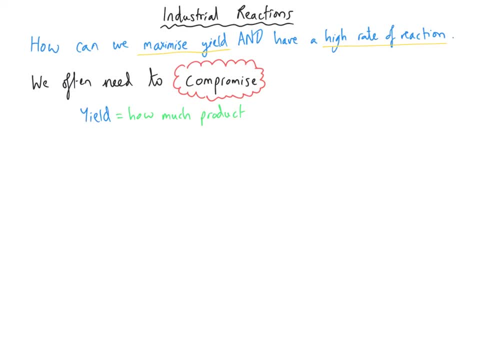 between the amount of product that we make, which is the yield, remember, and how quickly we get that product, which is the rate of reaction. And something to note from the get-go is 100% yield. if it takes a month is not as good as 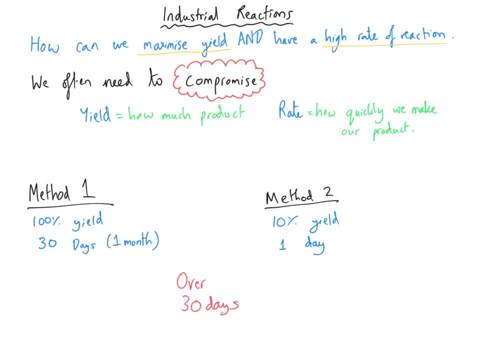 a 10% yield if it takes one day, because over a 30-day period, in method 1, you get 100% yield, which sounds good, But in method 2, you get a 10% yield every day for 30 days. 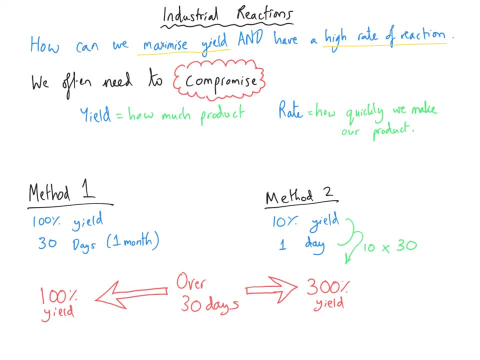 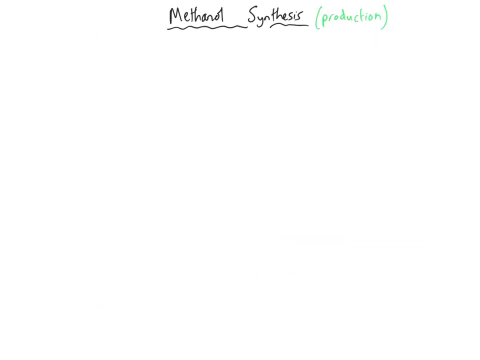 so that's 300% yield for purposes of comparison. So method 2,, even though it sounds less good on paper, it gets us three times the amount of product over the same period of time. The first industrial process we're going to look at is the synthesis, or production. 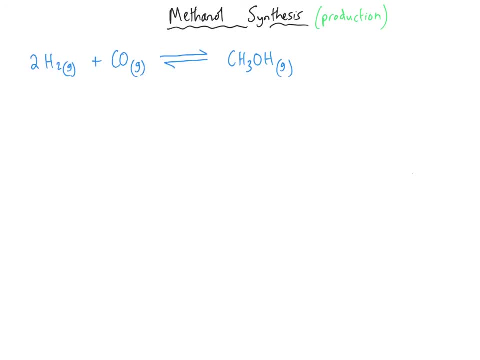 of methanol, from hydrogen gas and carbon monoxide, And so this reaction, as you can see from the equation here, involves three molecules of gas turning into one molecule of gas, and the forward reaction is exothermic. And so we can use our knowledge of Le Chatelier. 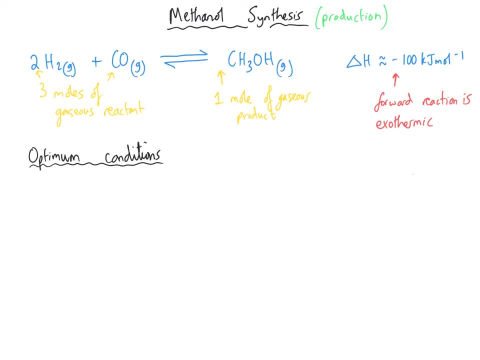 to work out what the optimum conditions would be to maximise the yield of methanol. So we need to think first of all about what we want the equilibrium to do. Whatever we do to the chemicals, however, we manipulate the conditions. we want to make the equilibrium 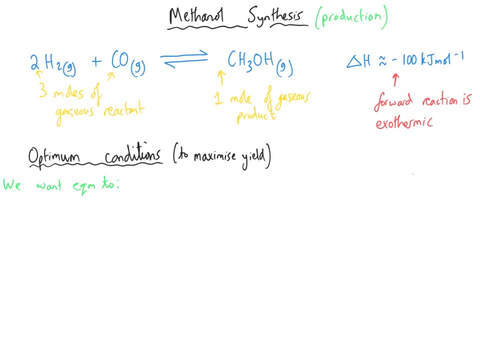 shift to the right hand side, So the equilibrium needs to be shifting in the forwards direction. Now, the forwards direction involves an increase in temperature because it's exothermic when we look at that delta H value, And so it would follow that 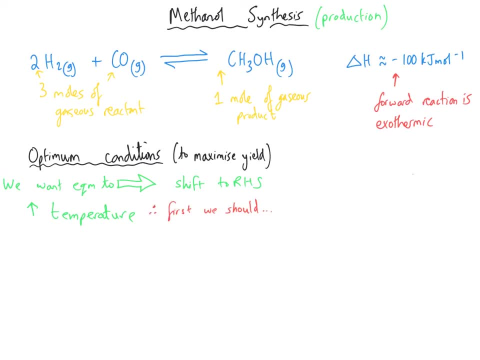 if we want the equilibrium to increase the temperature before it does it, we need to first lower the temperature and have a low temperature reaction, And that would favour the equilibrium shifting to the right. Also, the forward reaction involves a decrease in pressure, because the right hand 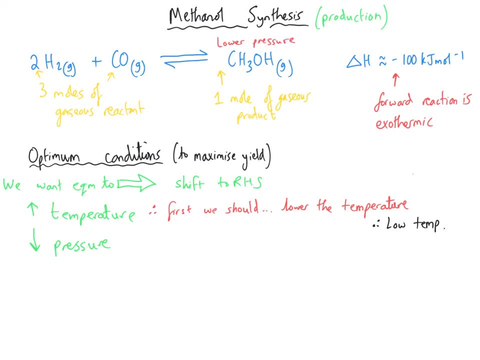 side is lower pressure than the left hand side, And so to make the equilibrium shift forwards, to decrease the pressure, we first need to have a higher pressure to maximise the yield of methanol. Now, in practice, we use a high pressure, about 50 to 100. 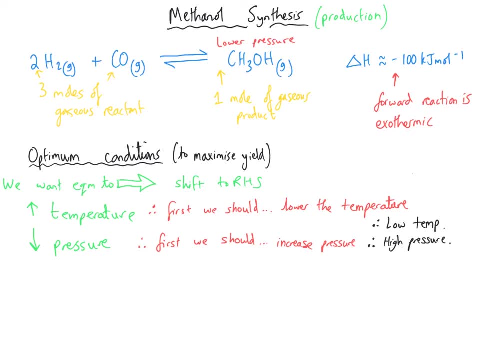 atmospheres. so that means about 50 to 100 times higher pressure than atmospheric pressure, And that gives us both a good yield and a fast rate of reaction. We use a temperature of 250 degrees C, which is not low but from an industrial point of view. 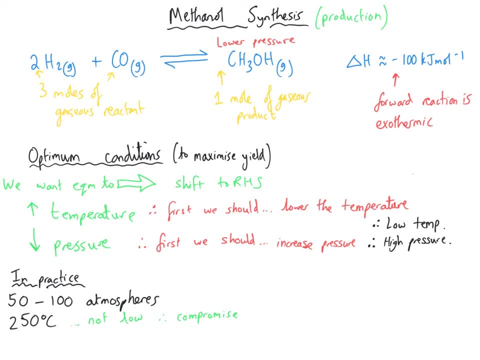 it's not a high temperature And that's because we want to try and maximise yield. remember, we'd ideally want a very low temperature, but we don't want to compromise on rate of reaction Because, remember, a higher temperature is a faster rate of reaction. 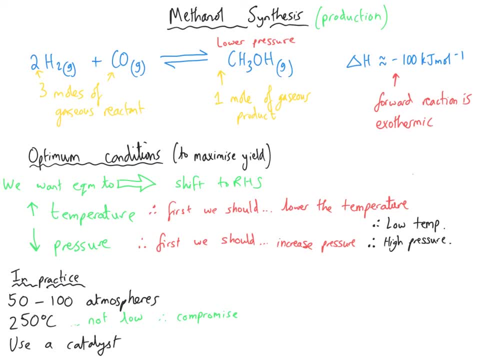 And so, to make up for the fact that we are compromising on the rate of reaction, we include a catalyst which is a mixture of copper, zinc oxide and aluminium, And that helps us to get over our compromise that we're having to do. 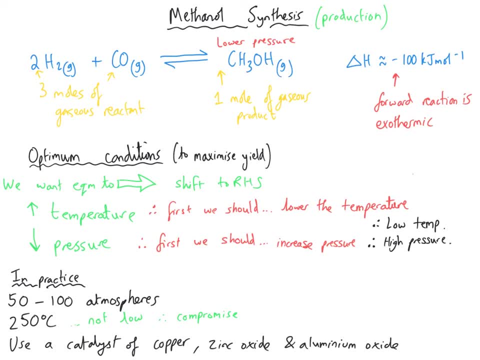 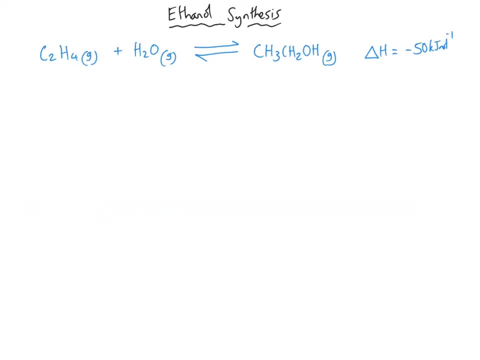 So we're trying to keep the temperature as low as possible without reducing the rate of reaction too much. Another industrial process you need to know about is the synthesis of ethanol, which we explore also in the alcohols video. So check that out sometime. 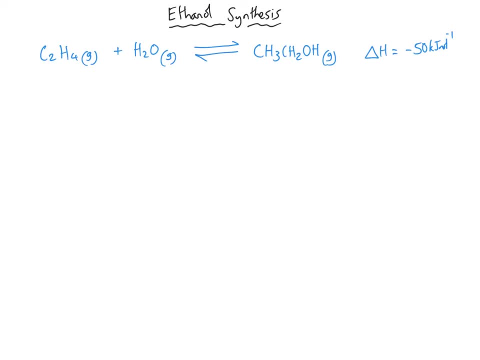 In the industrial synthesis of ethanol, which does not come from renewable materials, we use ethene gas and steam and that gets converted into ethanol in an equilibrium reaction that is exothermic. Now, in the same way as for methanol, let's look at 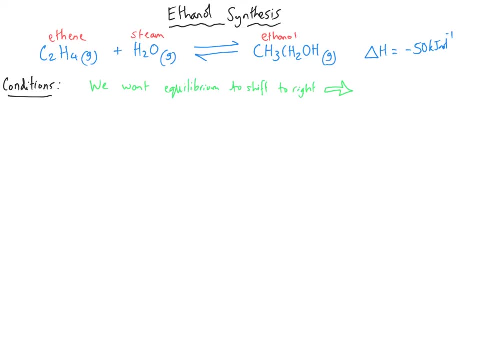 what conditions would favour this reaction? So, because we've got two moles of gas on the left hand side and one on the right hand side, we want equilibrium to shift in the forwards direction, which decreases the pressure. so ideally we would want to use high pressure. 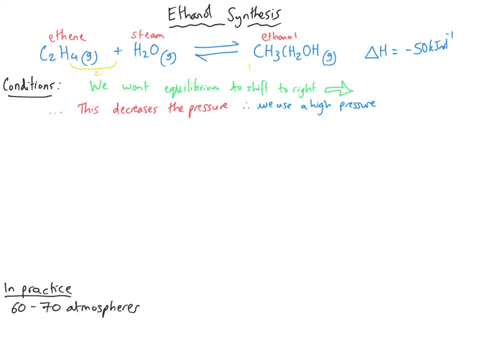 And in practice we use quite a high pressure, 60 to 70 atmospheres, so a little bit lower than for the methanol synthesis. And the reason for that is that at high pressures the ethene actually tends to polymerise to polyethene. 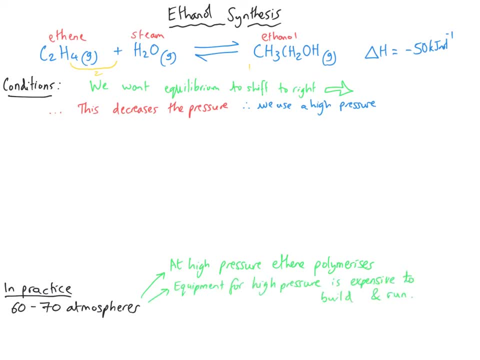 And also it's really quite expensive to build a power plant that can generate a high pressure and also it costs quite a lot of money to run the high pressure apparatus. So 60 to 70 is a slightly different kind of compromise and it's not simply about 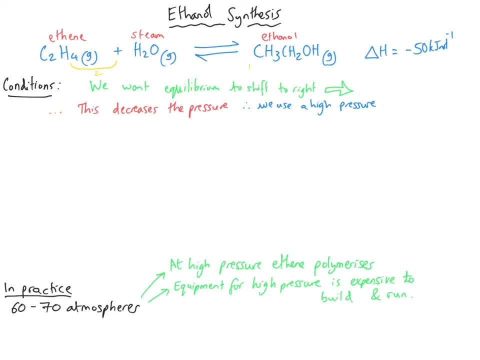 the rate, Although, because we're compromising on pressure and therefore rate, we do use a catalyst, which is phosphoric acid, most commonly. Now, in terms of temperature, once again, the forward reaction is exothermic, so we want the equilibrium to go to the right hand side in the direction. 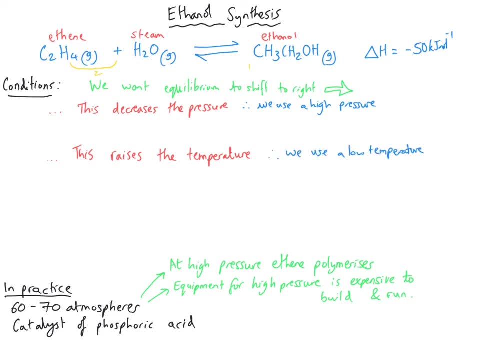 that raises the temperature. so in theory we should use a low temperature because that would maximise our yield, But because we're compromising already on pressure, lowering the rate of reaction, that way we actually use a temperature of 300 degrees C, So similar. 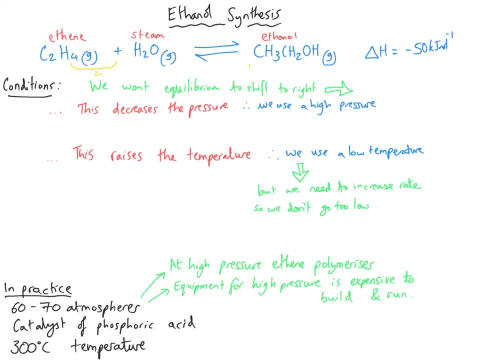 to the methanol temperature, but a little bit higher Once again, because we're compromising on the speed of the reaction. we have to therefore do something which wouldn't give us the biggest possible yield by having a higher temperature, But it's all a compromise where? 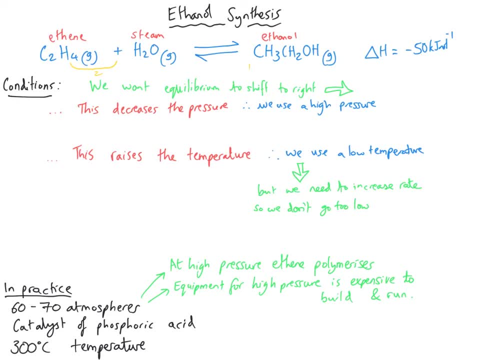 a variety of factors lean into each other: Safety, money rate and yield- all leading to these conditions, which do give us around 95% of ethene eventually converted into ethanol. One additional aspect of the practice is that, even though the yield is not 100%, 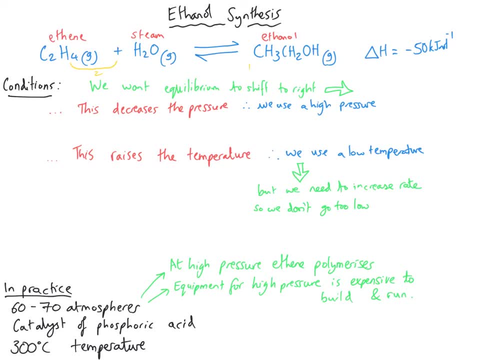 we get closer to it- 95%- by recycling the unreacted ethene, so that can go into the reactor again and again, And that's another way that we can push it up to 95% yield. One final process that we're going to look at is the 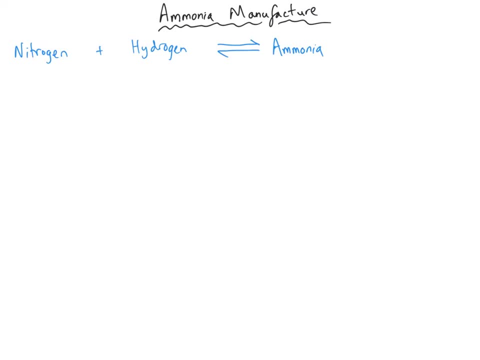 manufacture of ammonia. Now, I wouldn't normally ever give an A level student word equations, but the reason I'm doing that is because I want us to discover some things about the synthesis of ammonia from a graph, And so in exams they often give you. 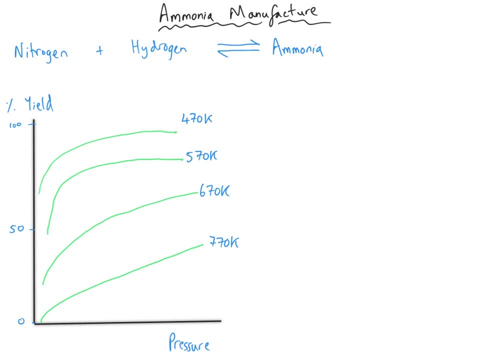 graphs for you to either interpret in a short term sense or give detailed analysis. So let's look, for example, first of all at general patterns on here. So we've got on the graph, as we increase the pressure going from left to right, the percentage yield of ammonia. 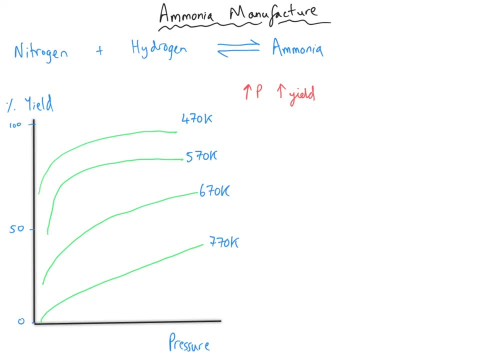 increases. So as we increase the pressure, the percentage yield goes up. All of these are different forms of sort of positive correlations. So because yield increases when pressure increases, we know that the forward reaction involves a decrease in the number of molecules of gas. 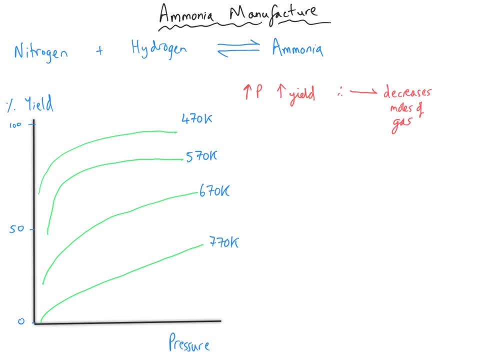 because that is the only explanation for a higher pressure, making the equilibrium shift to the right hand side, because the forward reaction must lead to a lower pressure. The other clue that we've got is we've got four separate lines on our graph at different temperatures, and we can see that the 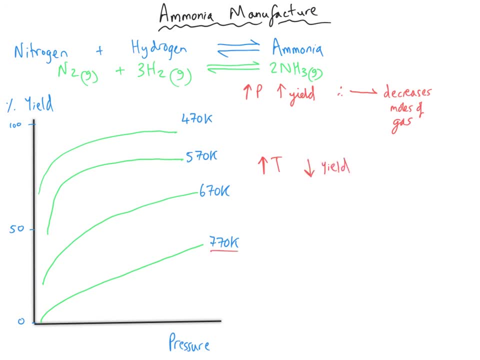 highest temperature gives us the lowest yield at the same pressure. So if we consider one particular pressure, let's say this pressure here- the yield for the 770 Kelvin is significantly less than for the other temperatures for the same pressure. And so because the greatest yield 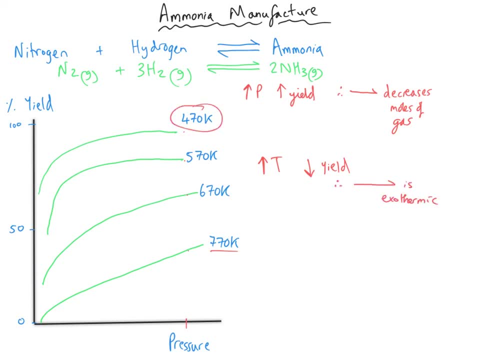 is found for the lowest temperature. that must mean that the forward reaction is exothermic, because a high yield is favoured by a lower temperature. So the lower the temperature, the more the equilibrium is able to shift to the right hand side. to maximise that, 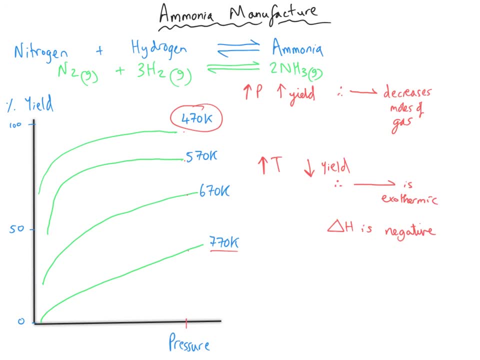 yield. So we can look at this graph to deduce that the forward reaction involves a decrease in moles and involves an exothermic process. We can also use this graph in a bit greater depth to make some suggestions about the temperature and the pressure that we should use, or to 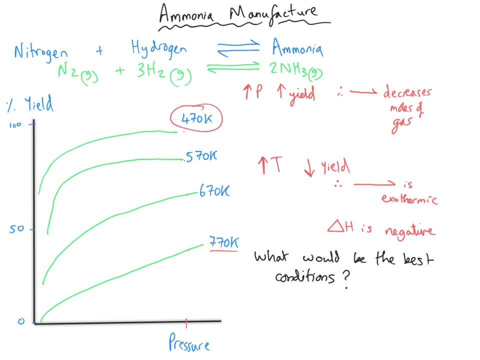 justify the pressure. So, for instance, if we look at the top line after maybe this pressure here, there is no point increasing the pressure any further because that will be really expensive and there's very little difference in rate of reaction in this entire tracking on here. It's not quite flat.